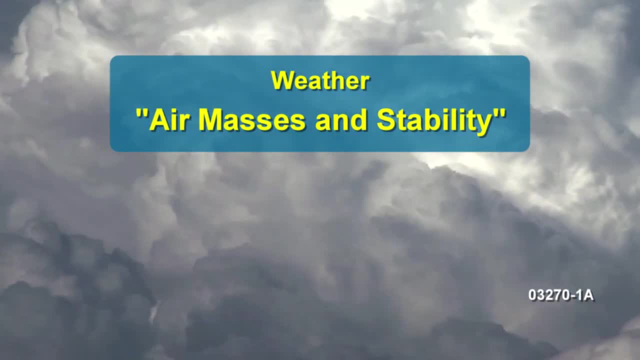 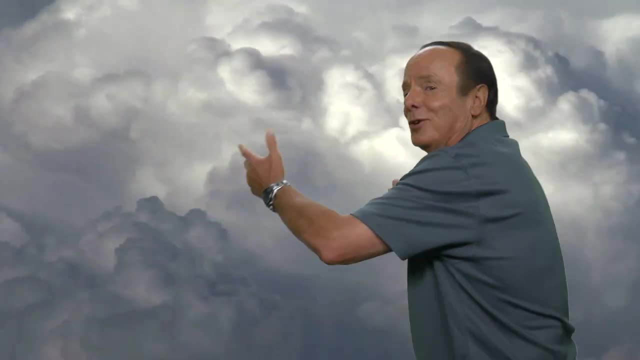 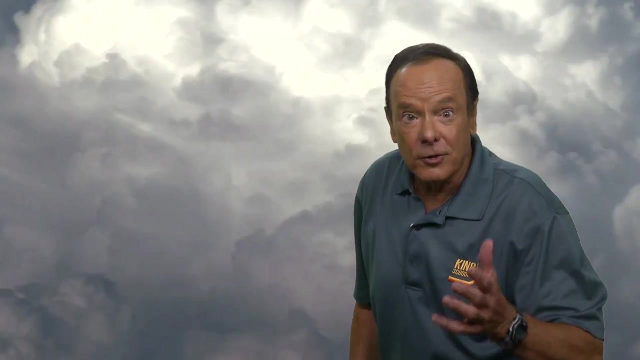 You know, as an instrument-rated pilot, the weather is a big deal to you, So let's talk about some basics about the weather that you'll use for the rest of your flying career. Now, the first thing you want to know is that the primary cause of weather changes is unequal heating of the Earth's surface. 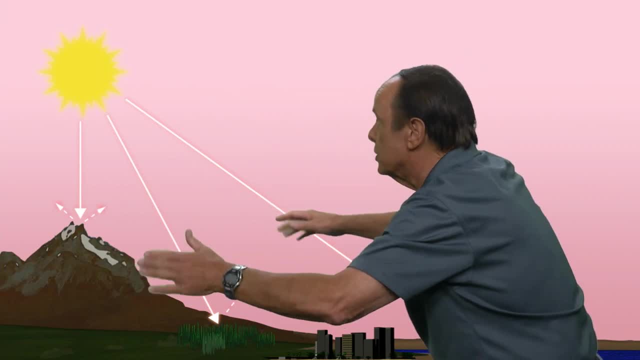 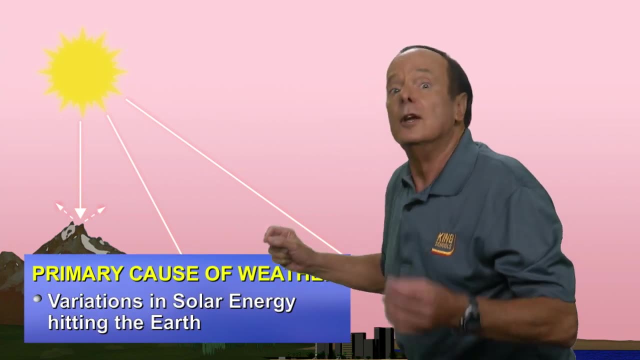 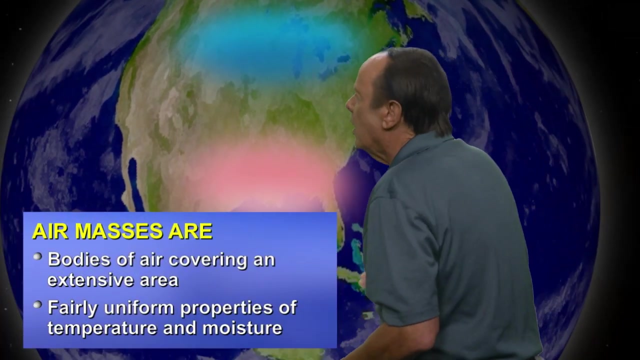 You see, the amount of the sun's energy, or what they call solar energy, reaching the surface varies in different regions of the Earth, And it's those variations in solar energy that cause the changes in the Earth's weather. It's also important that we know about air masses. Air masses are large bodies of air that cover extensive areas of the Earth's surface. 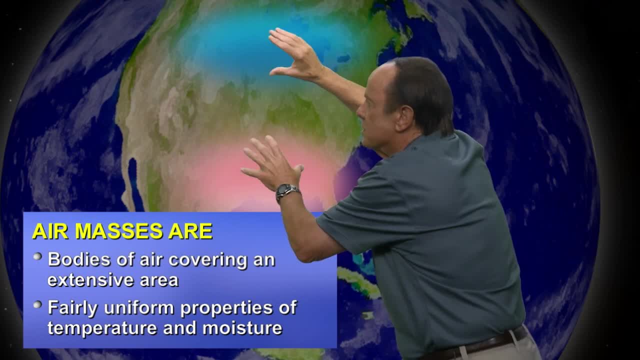 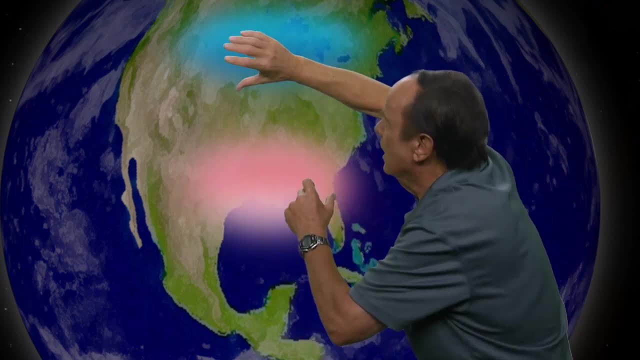 and they have fairly uniform properties of temperature and moisture inside them. Now, not all air masses are created equal. Some air masses are warm and humid, and others may be cold and dry, And the boundary between those air masses can cause all sorts of havoc. 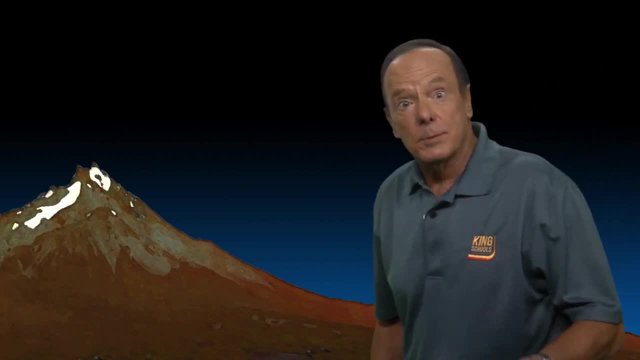 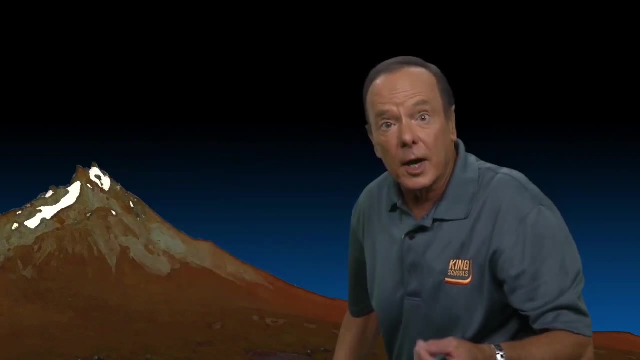 Now here is another thing you'll want to know about the atmosphere, And that is when you go to higher altitudes, the air cools off, And that's because, as you go to higher altitudes, there's less air pressure and the air expands. 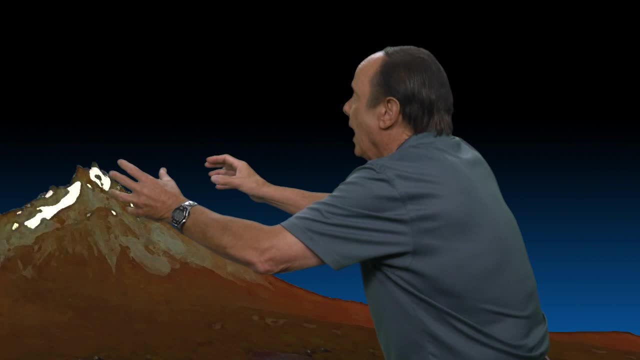 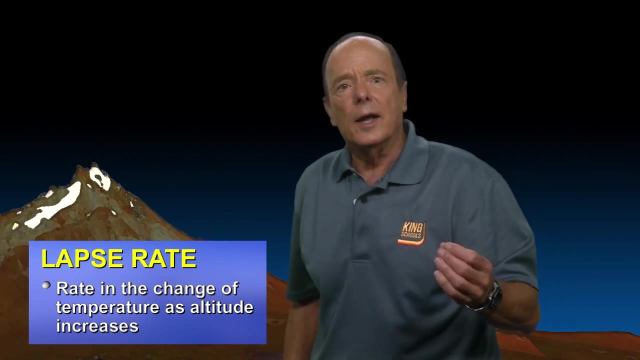 And as the air expands, it cools down, And the rate and change of the temperature as you go up, as you go to higher altitudes, is called the lapse rate. Now, if the air is dry, or what is called unsaturated, without any visible moisture, 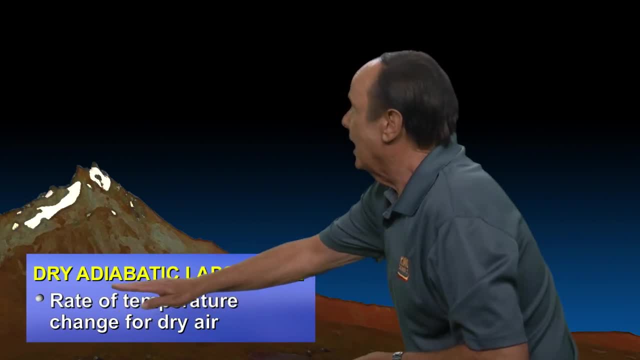 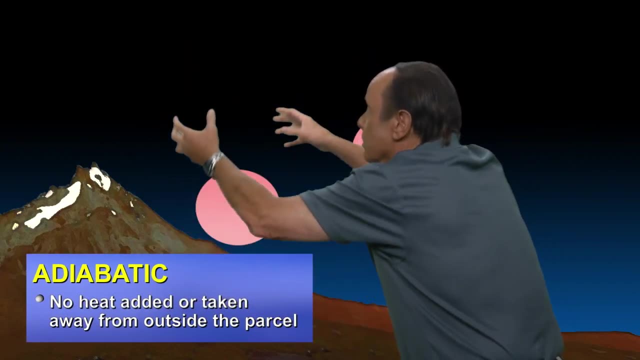 the rate at which the air cools down is called the dry adiabatic lapse rate. Now, adiabatic means that no heat is being added to or taken away from that parcel of air as it moves up and down through the atmosphere. 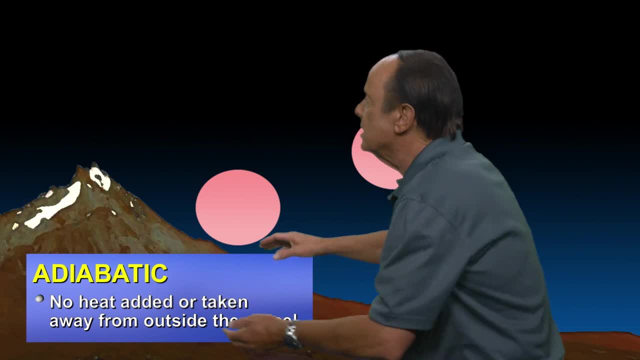 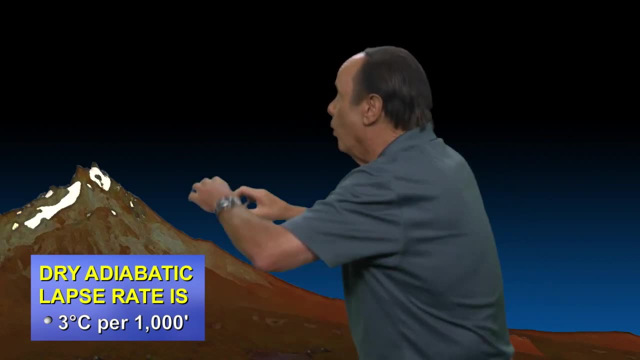 Now the dry adiabatic rate is 3 degrees Celsius for each 1,000 feet of altitude. change Now. eventually, as the air cools off, it will become wet or saturated, which means just the air can't hold any more moisture. 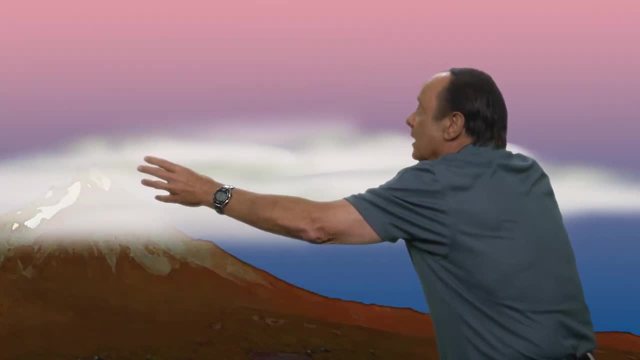 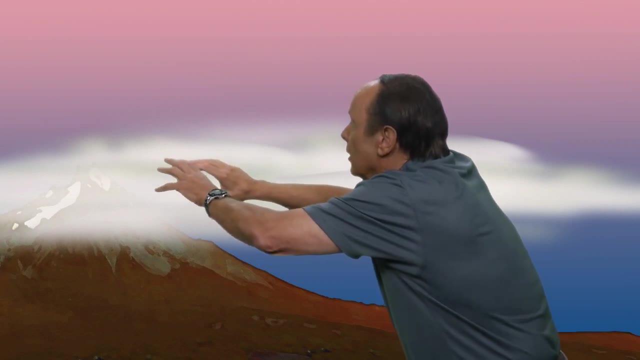 And when that happens, visible moisture forms, causing that lapse rate to change. And the reason for that is, as the air cools, water converts from a vapor state to the liquid state and gives off what is known as the heat of condensation. 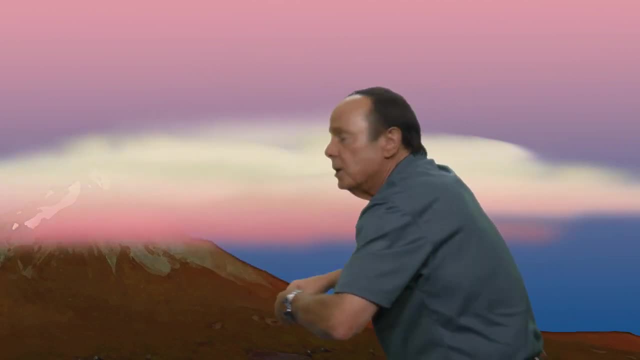 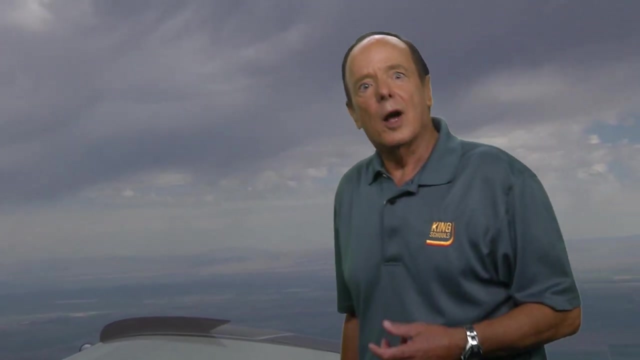 And that added heat prevents the air from cooling off as much as it would have if it were unsaturated. So when there's moisture in the air and the air becomes saturated, the lapse rate decreases because the air cools off slower. Now scientists, using average conditions from around the Earth 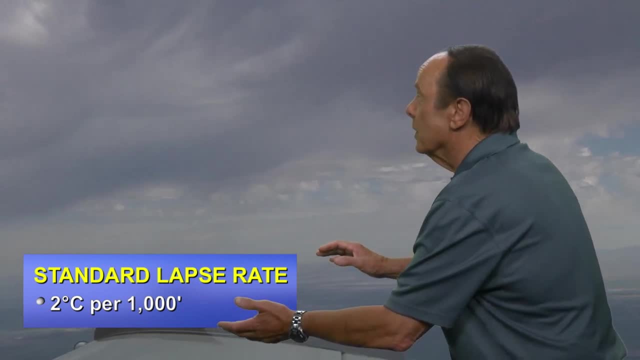 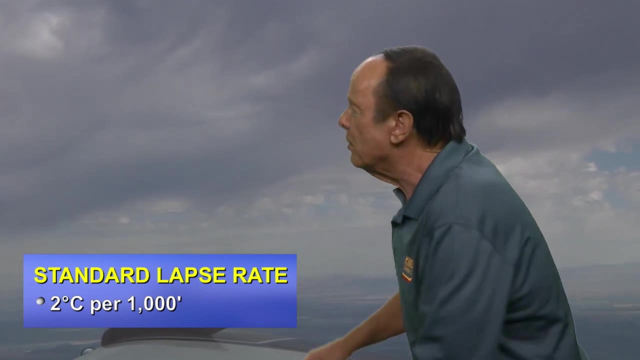 have determined what is known as a standard lapse rate, which is 2 degrees Celsius for each 1,000 feet that you go up. So let's take a look at a couple of ways that you might use this in your flying. First of all, you can determine how stable the air is. 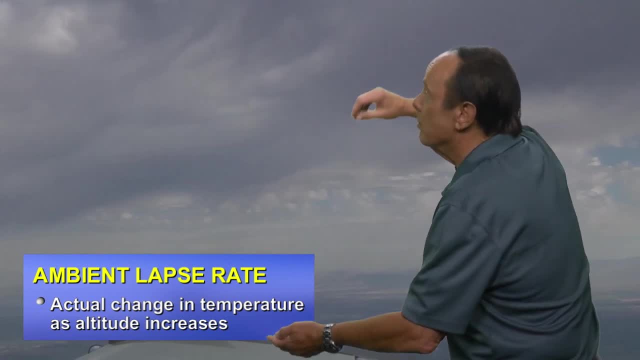 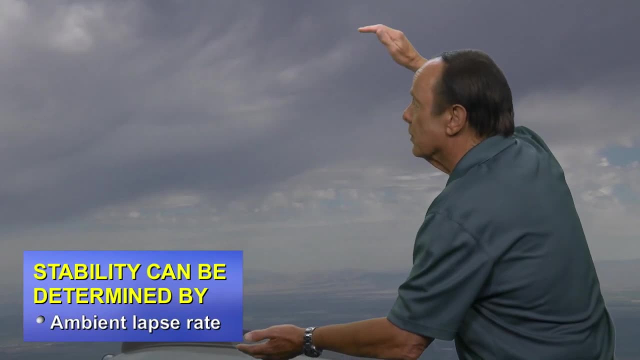 by knowing the actual lapse rate as you go to higher altitude compared to the standard lapse rate. So if you look at the actual lapse rate, or, as the FAA may call it, the ambient lapse rate, and then compare that to the standard lapse rate, 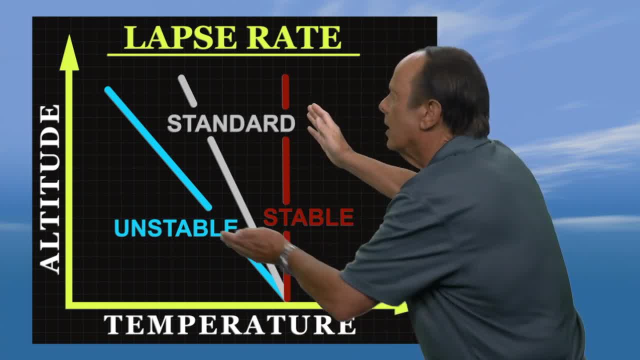 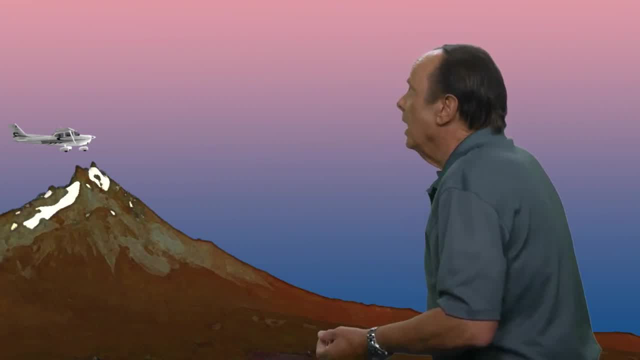 you'll know whether an air mass is likely to be stable or unstable, and if your flight is going to be a smooth or a bumpy one. Now, a stable air mass is one in which the air at higher altitude is much warmer than it would be if there were a standard lapse rate. So when a partial lapse rate occurs and a partial error is forced to rise in a stable air mass, it becomes colder and heavier than the surrounding air and it resists rising and you'll end up with stratiform clouds and smooth air. 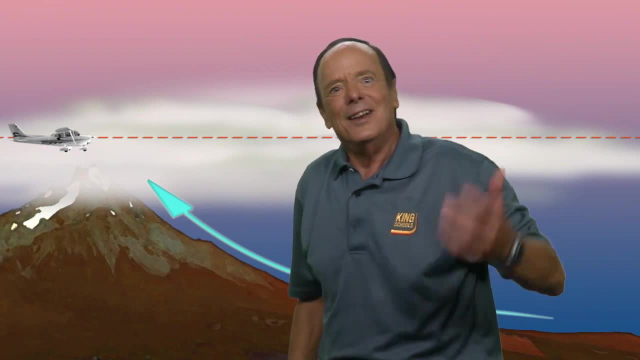 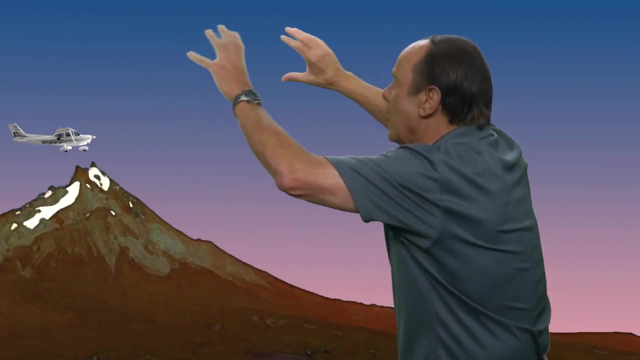 And all of us pilots sure like flying in smooth air. Now, an unstable air mass is one in which the air at higher altitude is much cooler than it would be if there were a standard lapse rate. Now, when a partial of error is forced to rise in an unstable air mass, 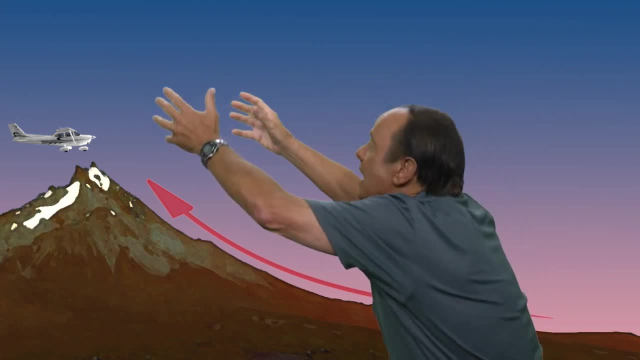 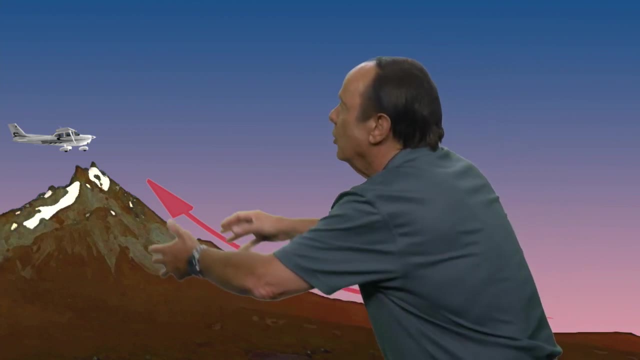 it becomes warmer and lighter than the surrounding air, and it keeps on rising. So what that means is that unstable air is air that is forced to go up and wants to continue to rise, And so you'll end up with cumulus clouds and a bumpy flight. 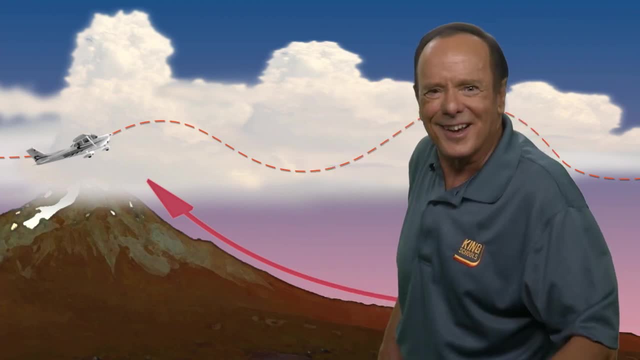 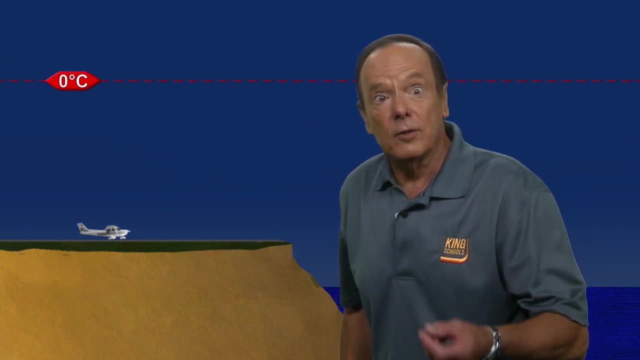 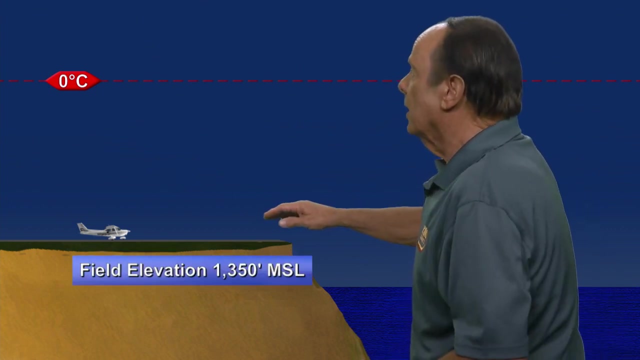 and neither you nor your passengers are going to appreciate that. Now, if you know the temperature of the air at the surface, you can also use the standard lapse rate to find out the approximate freezing level. Let's see how the math works. Let's assume that you're at an airport with an elevation of 1,350 feet MSL. 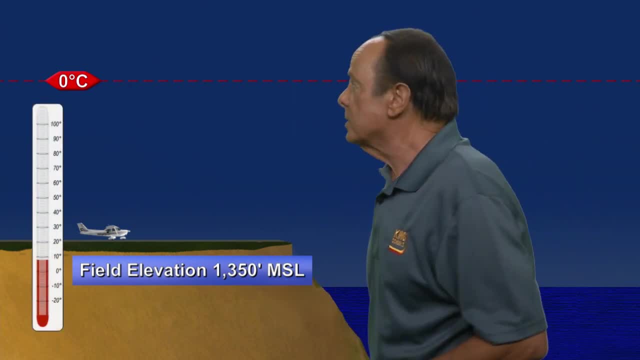 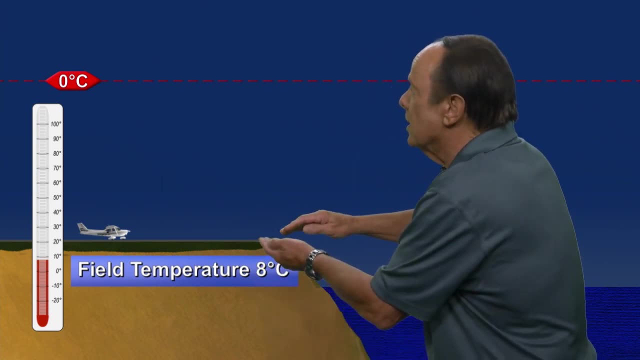 And let's assume also that the temperature at the airport is 8 degrees Celsius. Now we know that on a standard day the temperature cools off by 2 degrees Celsius for each thousand feet that you go up. So to find the freezing level. you take that 8 degrees Celsius divided by 2 degrees for each thousand feet, and that means the freezing level is about 4,000 feet higher. So if you climb up four more thousand feet, you ought to find a temperature of 0 degrees Celsius. 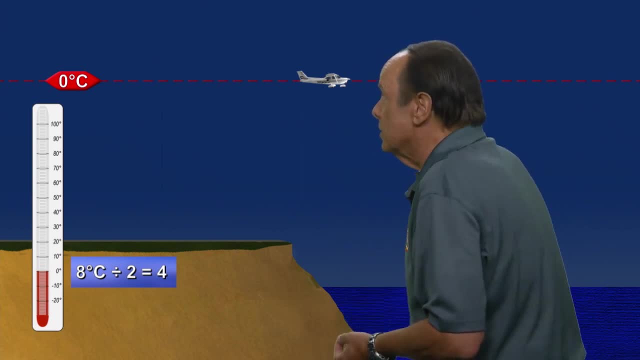 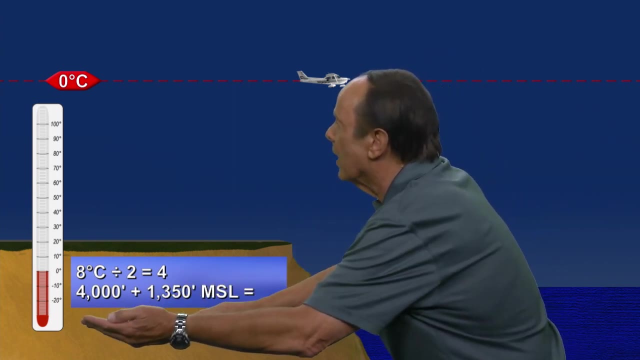 But originally we started this problem at a field elevation of 1,350 feet MSL. So you take that 1,350 feet MSL and add the 4,000 to it and you're going to be finding the freezing level of 5,350 feet MSL. 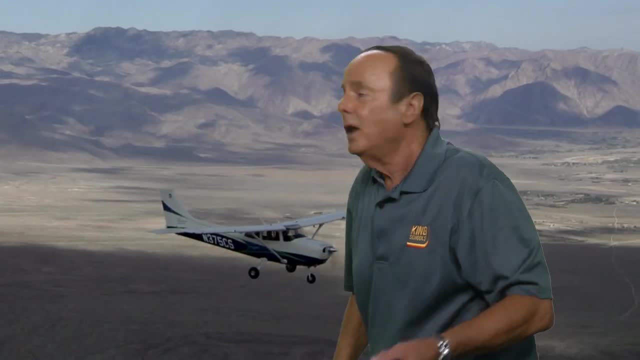 Well, folks, now you have some tools to help you plan a safer, smoother flight, And so that you and your passengers can land with a smile. 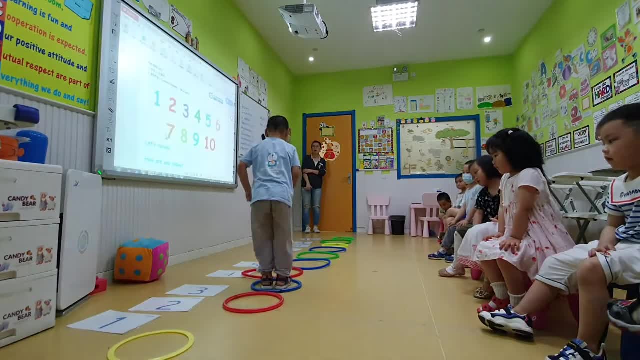 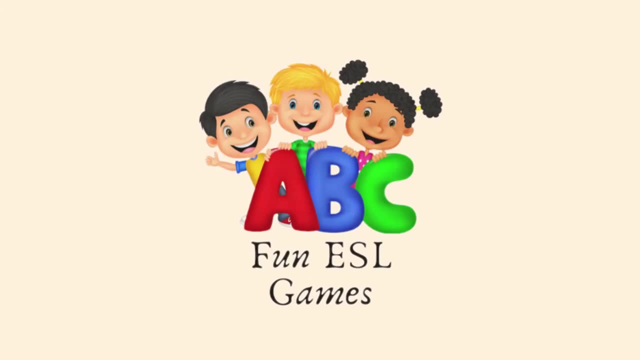 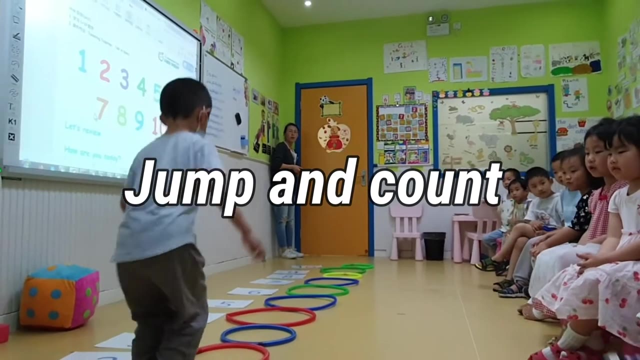 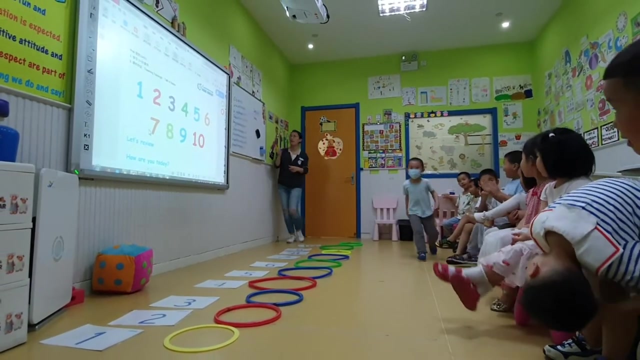 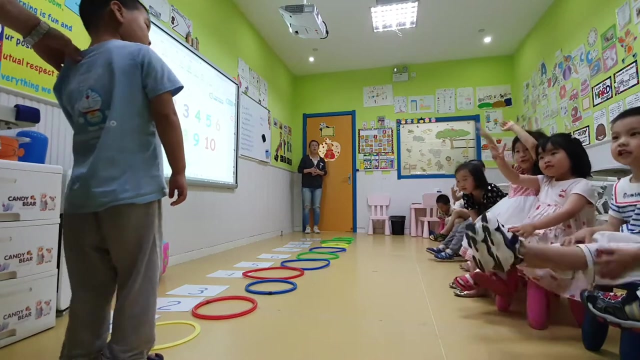 1,, 2,, 3,, 4, 5. 3,, 2,, 1, go. Oh, High five, high five. Yes, High five. what's that? 3,, 2,, 1, go. 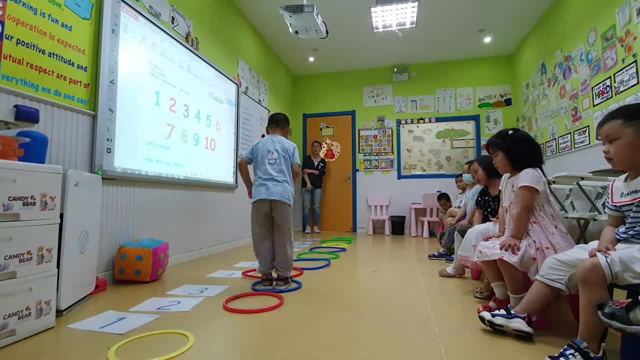 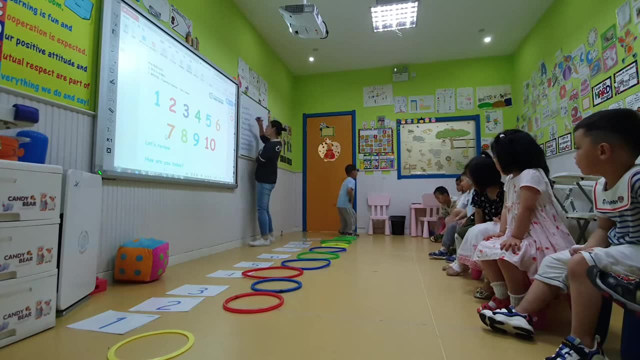 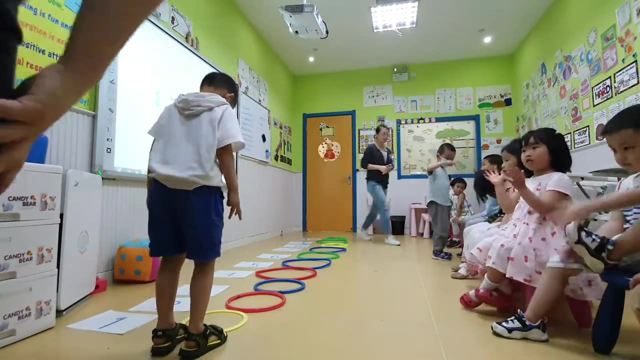 1,, 2,, 3,, 4,, 5,, 6,, 7,, 8,, 9, 10. Wow, Yes, Very nice. 3,, 2, 1, go. 1, 2,, 3,, 4,, 5,, 6,, 7,, 8,, 9, 10. 10,, 11,, 12,, 13,, 14,, 15,, 16,, 17,, 18,, 19,, 20, 20,, 21,, 22,, 23,, 24,, 25,, 26,, 27,, 28,, 29,, 30. 21,, 22,, 23,, 24,, 25,, 26,, 27,, 28, 30. 21,, 22,, 23,, 24,, 25,, 26,, 27,, 28, 30. 21,, 22,, 23,, 24,, 25,, 26,, 27,, 30, 21,, 22,, 23,, 24,, 25,, 26,, 27,, 30, 21,, 22,, 23,, 24,, 25,, 26,, 27,, 30.